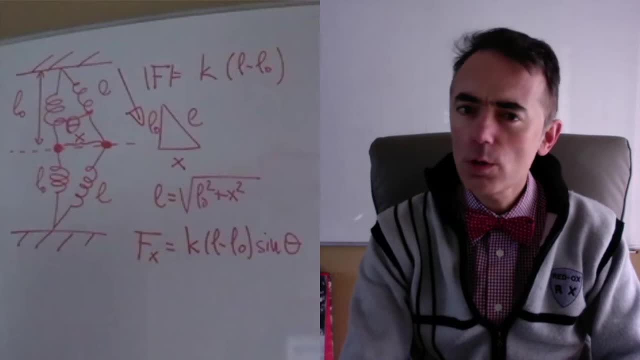 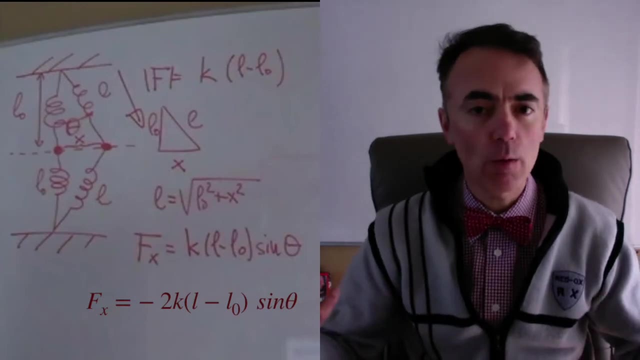 both springs point in the same direction. So the total x-axis force is minus 2KL, minus L0. sine of theta, Forces on the y-axis cancel out. But this force on the x-axis is written in terms of the stretched length and the angle. 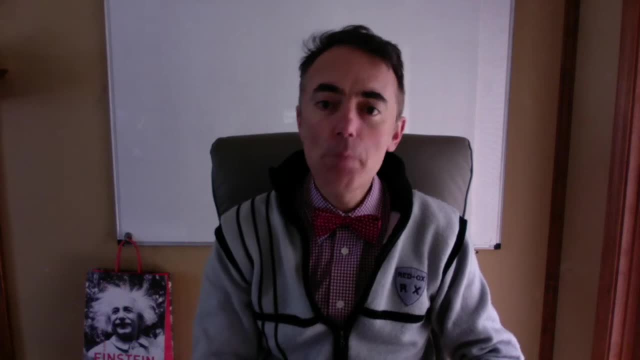 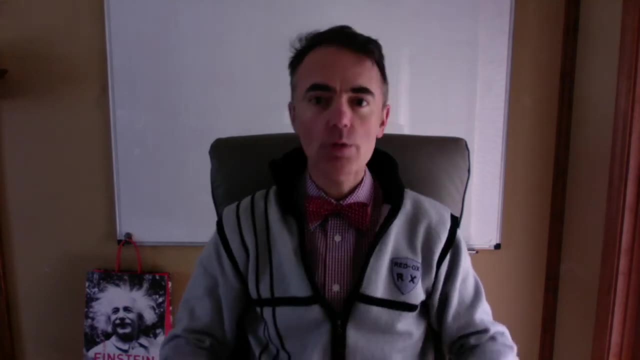 theta, both of which change in time And both of which are related. Let's write the force in terms of just one of these variables. To do that, I'll use trigonometry to write the sine of theta as the position x over L. 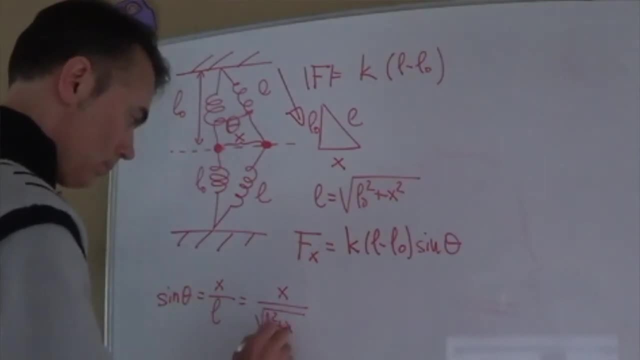 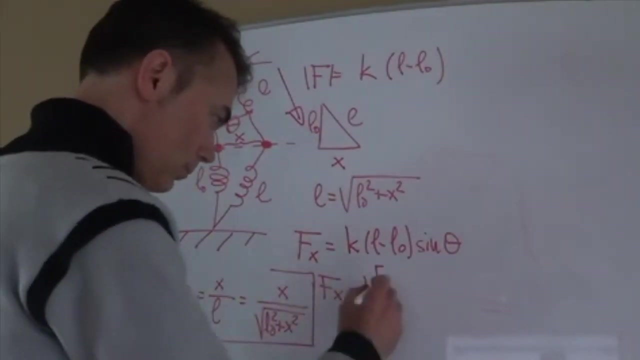 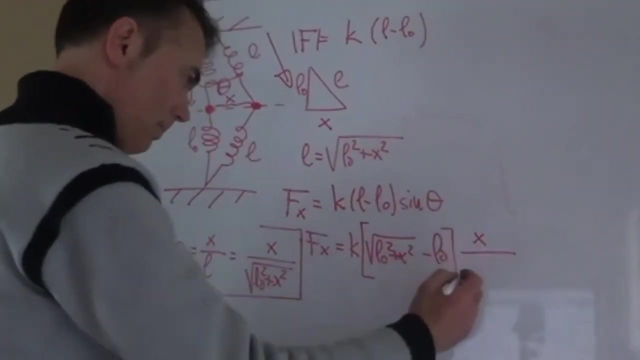 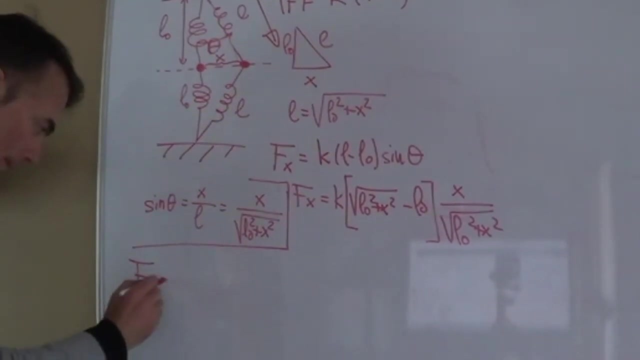 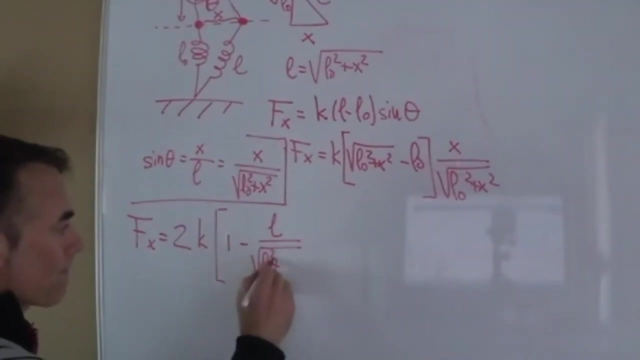 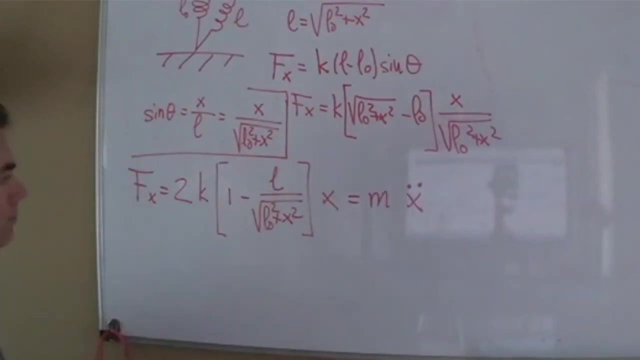 And I can write L as the square root of L0 square plus x square. This way I have the force written only in terms of x. This is not a very simple expression, though. Let's assume that the oscillations are small, and then this means that x over L0 square is. 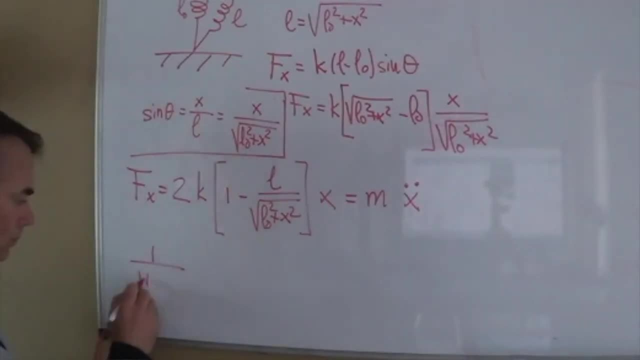 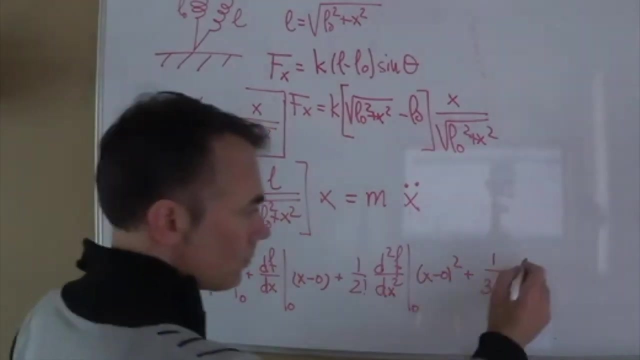 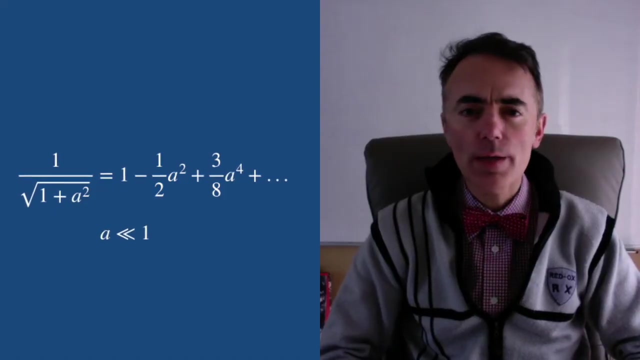 small. Let's expand this square root in series of Taylor. Remember that for a series of Taylor's expansion we approximate the function as the polynomial that we obtain by successive derivatives. So 1 over the square root of 1 plus a square for a very small can be approximated by 1 minus. 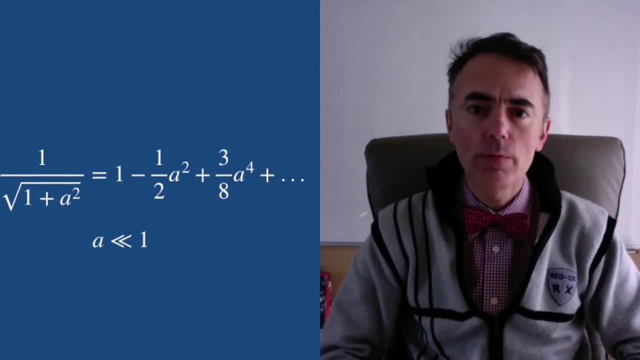 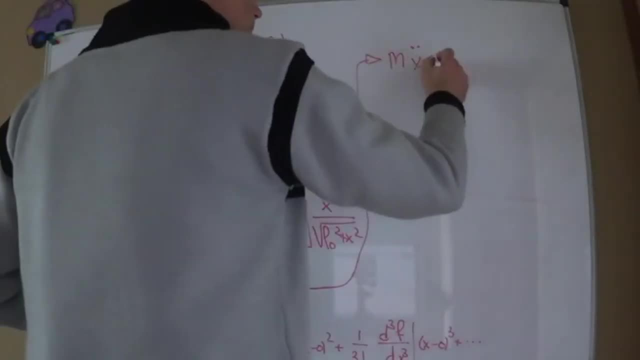 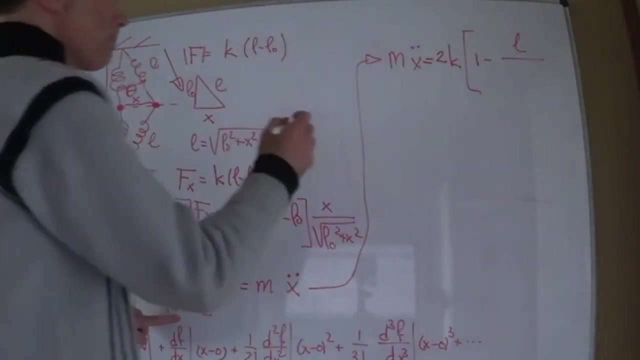 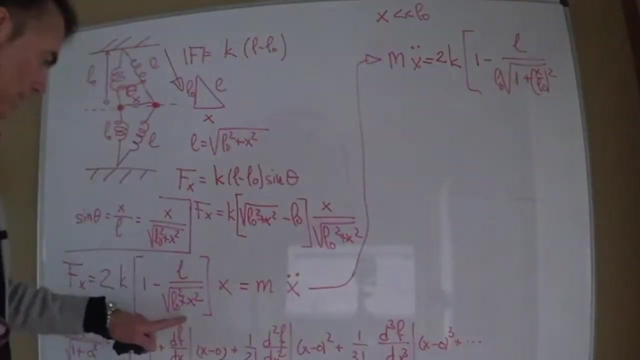 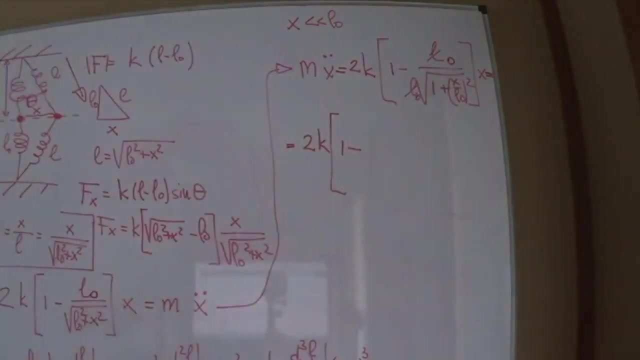 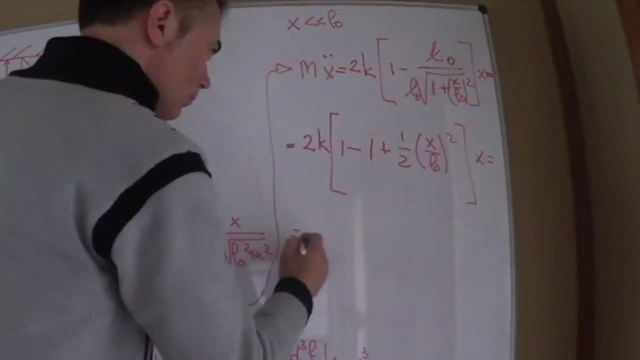 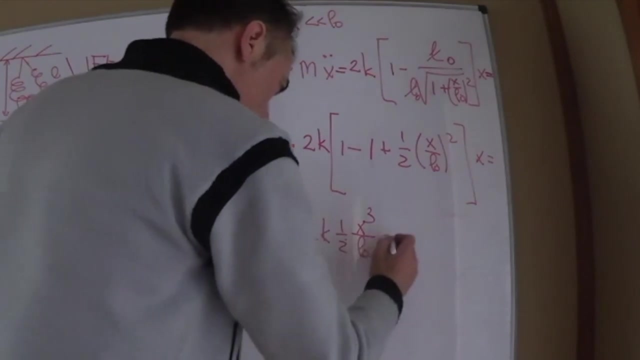 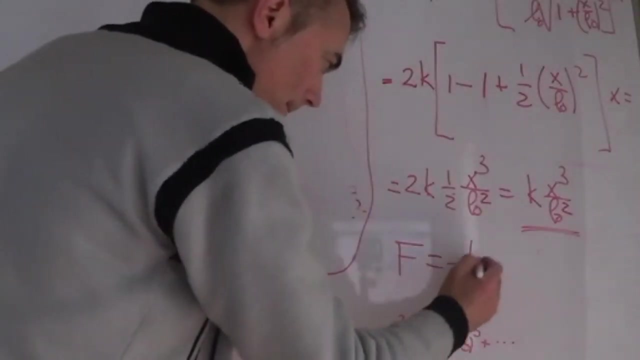 one half of a square plus 0.. 3 over 8 of a to the fourth. dot dot, dot This back into the force of the springs. this leaves us with this expression for the force on the mass. Look that the lowest term is to the power of 3.. 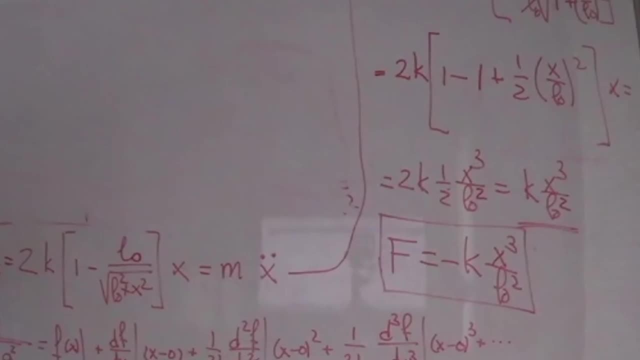 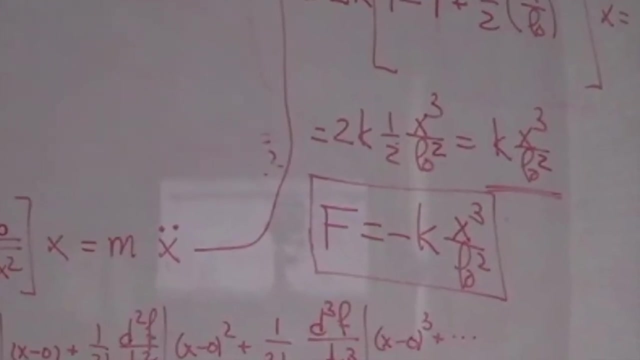 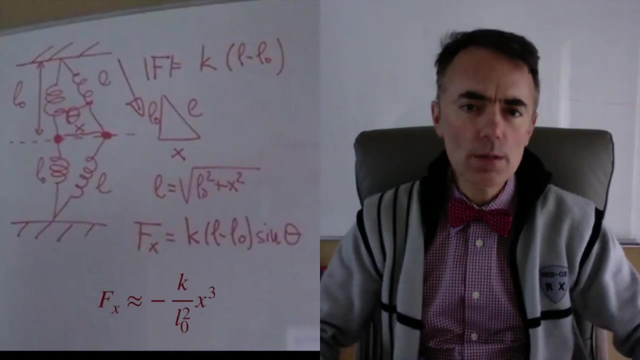 If we neglect higher order terms, we get, with f of x, approximately equal to minus k, over l0 square times x to the cube. This is a clearly non-linear force. This is not the simple case of Hooke's law, This simple system with only two springs attached to one mass. 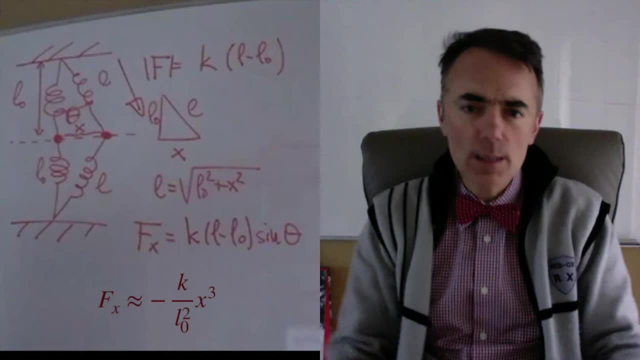 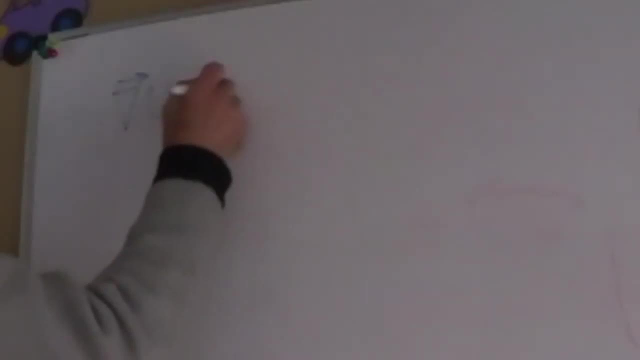 even for small oscillations, is an example of non-linear dynamics. We can find the potential related to this force, Using nabla of u, equal to negative- the force we integrate to get the potential- And it has a dependence of x to the power of 4.. 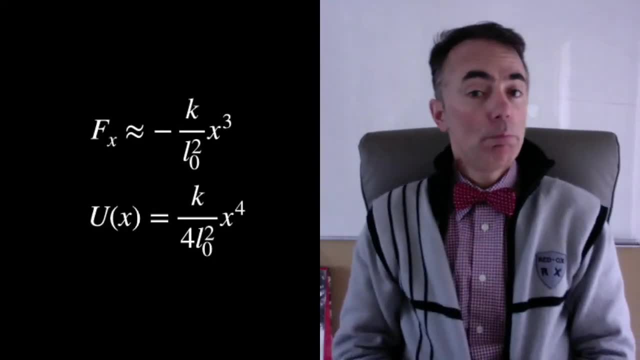 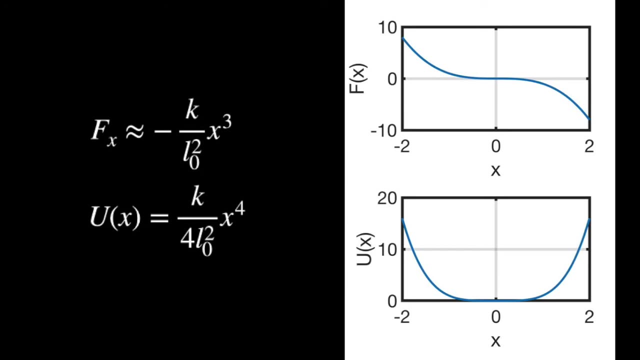 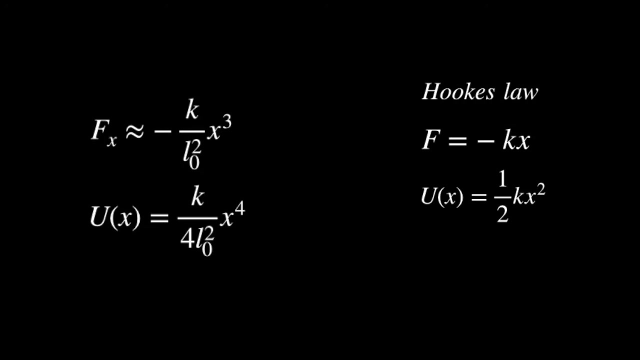 This is not a parabolic potential anymore. We can plot the force as a function of the position and the potential as a function of the position. Remember that in the case of Hooke's law, we had a potential in terms of x squared. 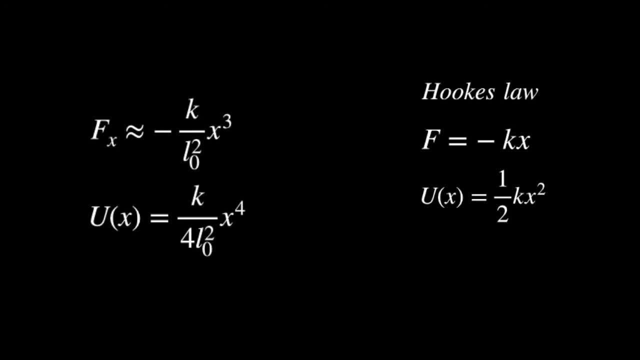 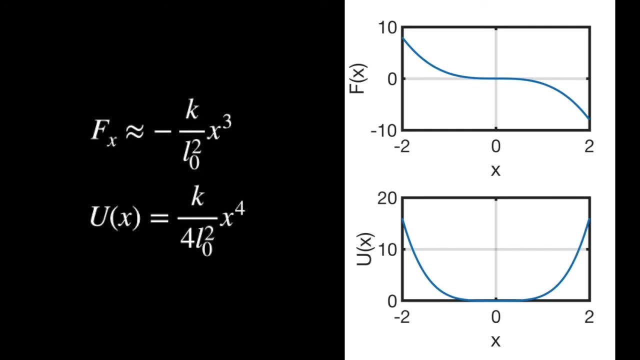 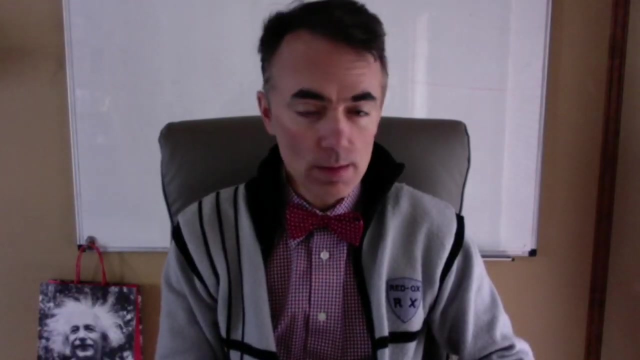 That was a parabola, But not here. This is still a symmetric potential, though The same happens for positive x as for negative x, But we can't use the quadratic approximation for the potential. We can also integrate this differential equation to find the velocity of the particle as a function of the position. 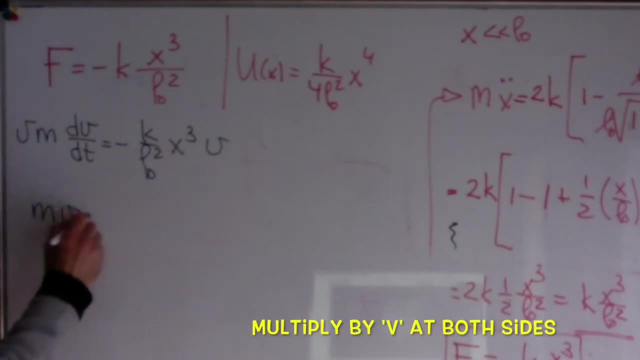 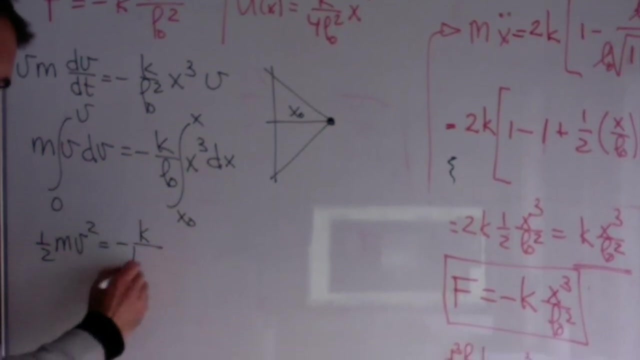 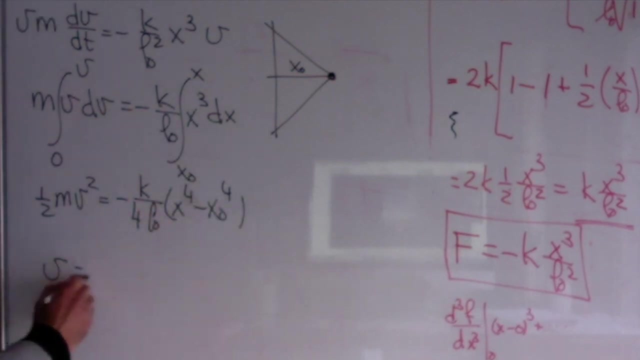 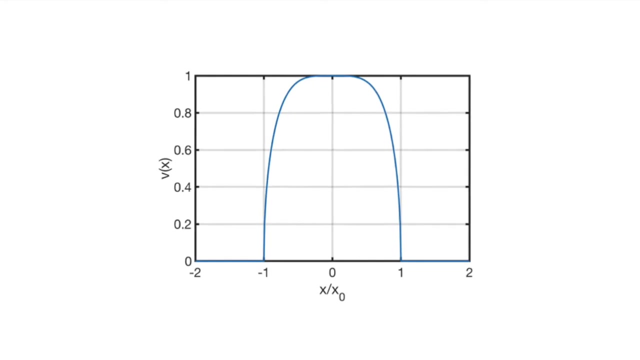 So we can use the differential equation to find the velocity of the particle. And now we can plot the velocity as a function of the position. And now we can plot the velocity as a function of the position. And now we can plot the velocity as a function of the position. 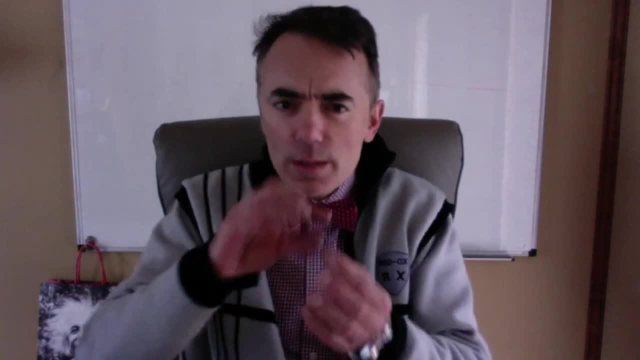 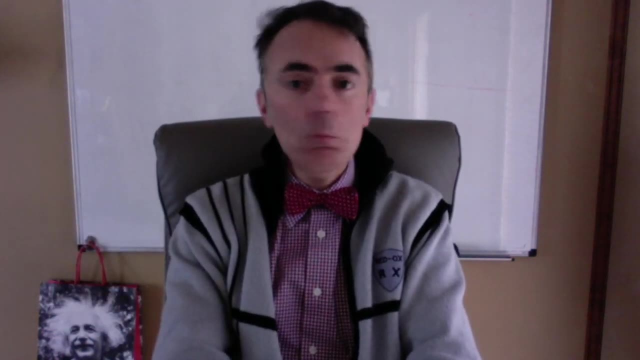 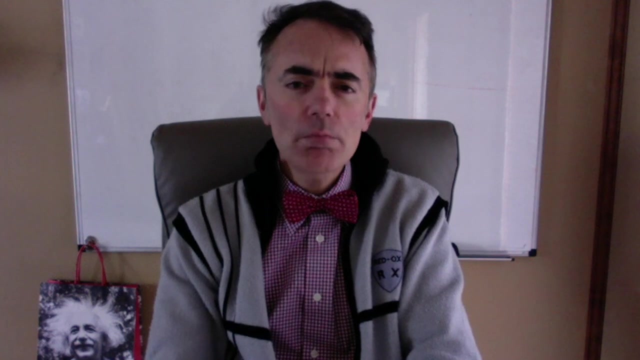 So something we can do now is to assume that before we start the motion the springs are already stretched. They are not in their equilibrium position. Then we repeat, We move slightly the mass from its equilibrium and let go. But this We'll solve in the next video. May the science be with you.